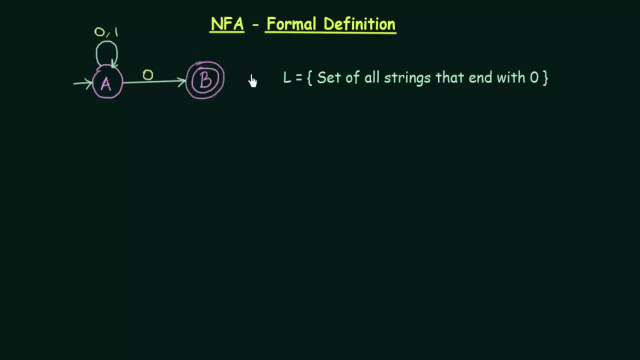 perfectly legal to leave a state like this without mentioning anything. that actually means that this state does not go anywhere, all right, which was not legal in DFA, but in case of NFA it is perfectly legal and this is a complete NFA, all right, and by looking at this, you can guess that it is very easy to design. it is very easy to design a NFA as compared to DFA, because in DFA, we 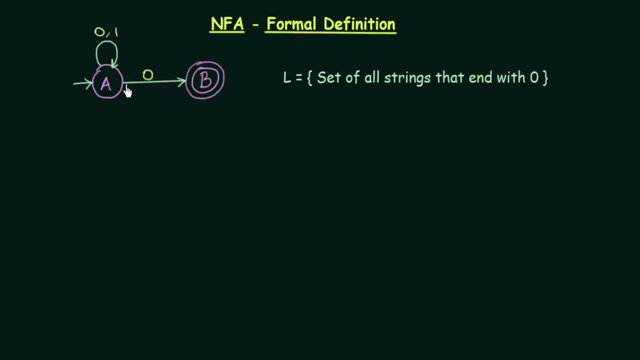 have to be very careful about sending the state standing the say states to only one next state and we should also mention clearly on getting input: whatever inputs they are, we should show what is a transition from each input. but in NFA we find that even if you leave it like this, it is complete. so it is very easy and 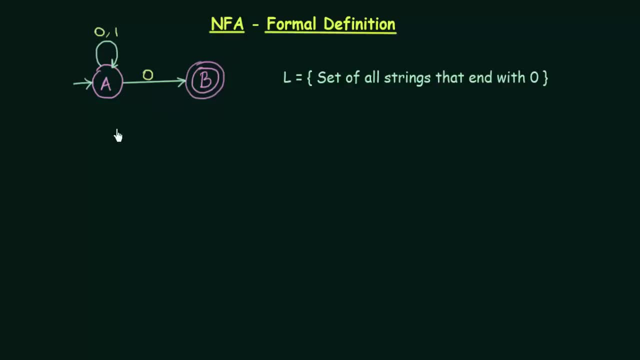 straightforward to design a NFA all right. now let us try to give the formal definition. so, just like DFA, NFA also is defined using five tuples, which are Q, Sigma, Q0, F and Del. Using these five tuples, we can define our NFA. 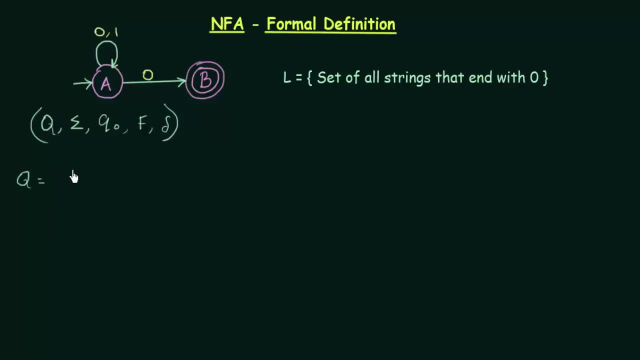 And what are these? Let me write it down. It is almost the same like DFA: Q is the set of all states and Sigma is the inputs, and Q0 is the start state or the initial state, And then F is the set of final states and Del. 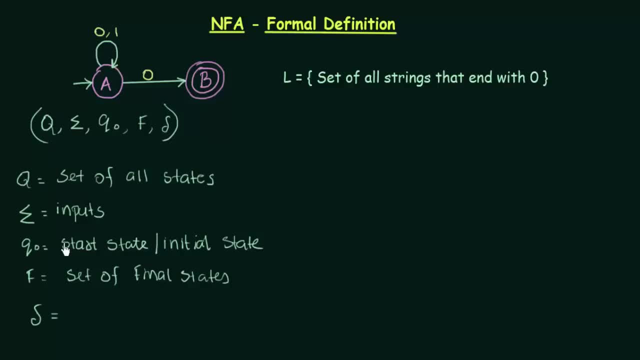 So we saw that this Q, Sigma, Q0 and F is same, like the DFA that we have already studied. And what about Del? Del is a transition function that maps Q cross Sigma to what. We will try to find out what this is. 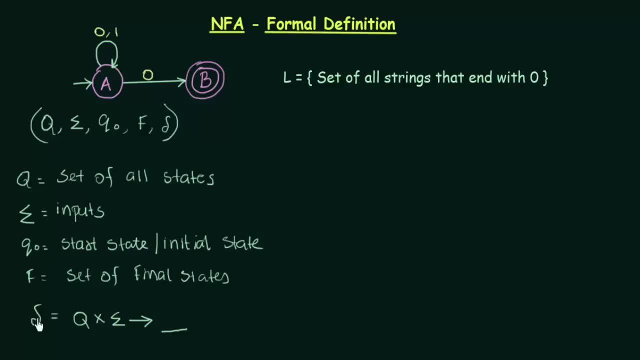 I will leave it blank here. We will try to find out. what does this transition function? Del map? Alright, that is what we are going to find out. Okay, so Q, Sigma, Q0 and F are the same like DFA, So I hope I don't need to explain it again. 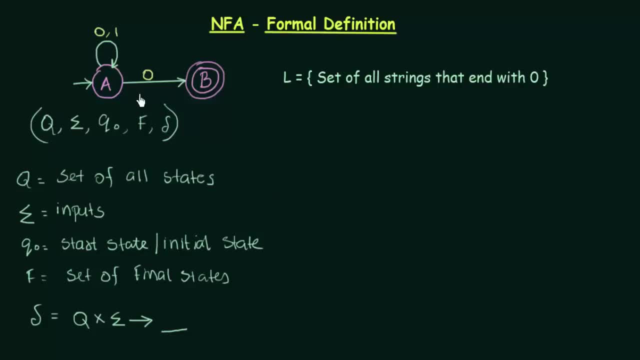 So let us just try to write down the values for this particular example. So in this particular example, what is Q? Q is the set of all states. So what are the set of all states? here, The only states we have are state A and state B. 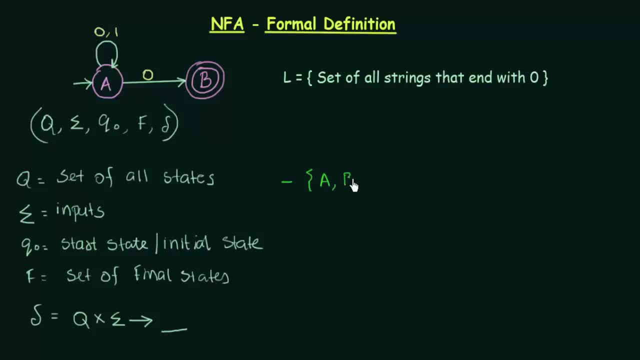 So it is A and B, Alright. and Sigma is the inputs. So what are the inputs we have? The inputs we have are 0s and 1s. The inputs are 0 and 1.. And Q0 is the start state or the initial state. 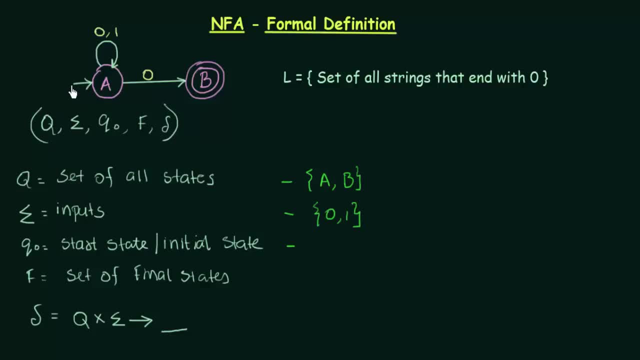 And how do we know which is the start state? The state that is pointed by this arrow coming from nowhere shows that this is the start state. So the start state is 0.. So the start state is A, which is also known as the initial state. 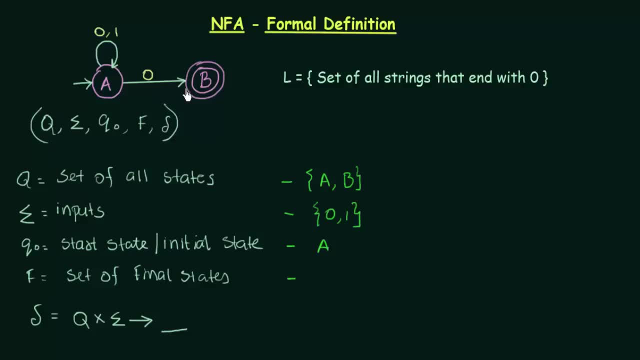 And what is F? F is the set of final states. So here we have only one final state, that is B, represented by the double circle. Now, what is del? How do we find out what is del? This is what we are going to find out. 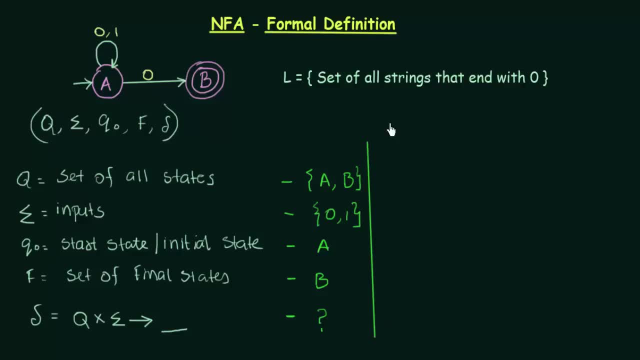 Okay, so when we try to find this out, let us try to do some exercise. Let us see, Let us check for state A, State A on getting input 0, where does it go? It goes to state A itself. And state A on getting input 0, it also goes to state B. 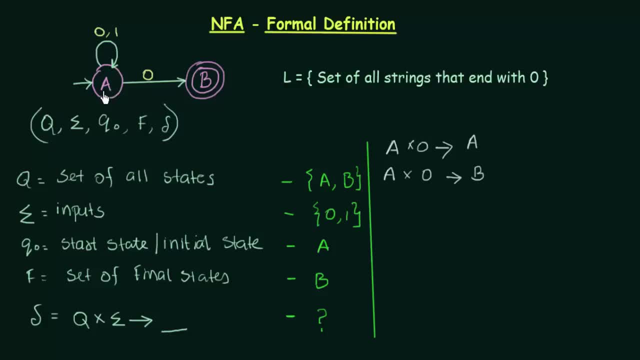 Alright, And let us see when state A gets input 1, what happens When state A gets input 1, it goes to state A itself. State A itself, Right? Yeah, that is it for state A. And what about state B? 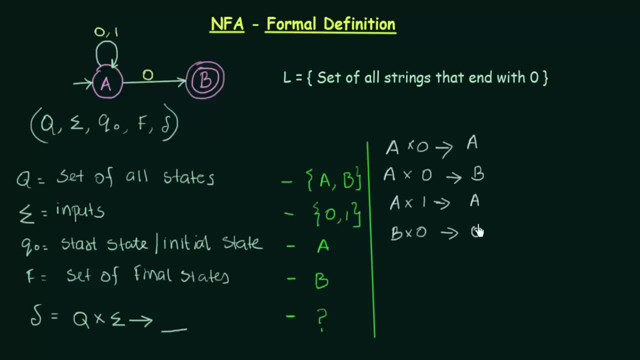 State B on getting input 0, where does it go? It does not go anywhere, So we represent it with 5.. Alright, And what about state B on getting input 1, where does it go? It again goes nowhere. 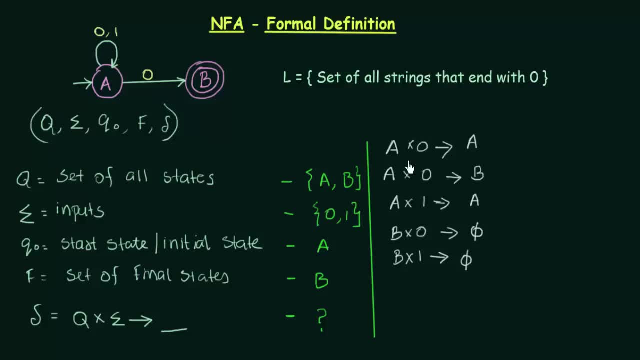 So it is again represented by 5.. So we see that, given a state, when it gets a particular input, it can either go to state B or state A, One state or more than one state. So we see that A on getting input 0, it went to two states, A and B. 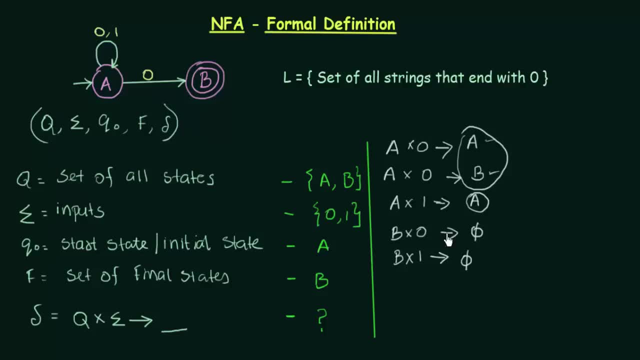 And A on getting input 1, it went to just one state. So there are many possibilities. Let us try to figure out how many possibilities are there. Suppose for this example A and B are there, And let us see what are the possibilities that we can get. 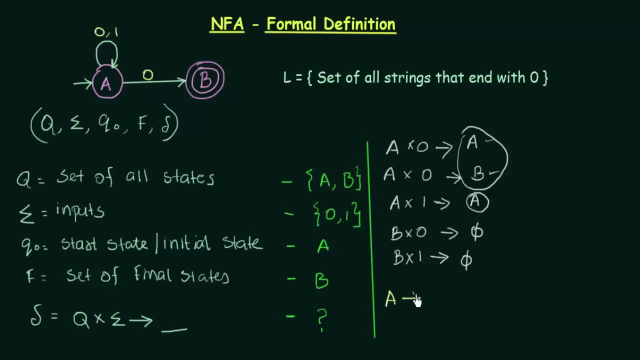 So let us talk for one state A: A on getting a certain input. let us say 0 or 1, whatever it may be. on getting a certain input, it can either go to A or it can go to B, or it can go to both A and B. 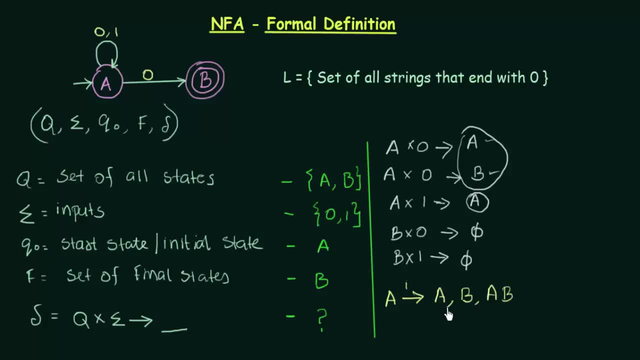 Like here, it went to both A and B. So it can either go to A, it can either go to B, or it can go to both A and B, Or it can also go nowhere, Just like we saw that B was going nowhere. 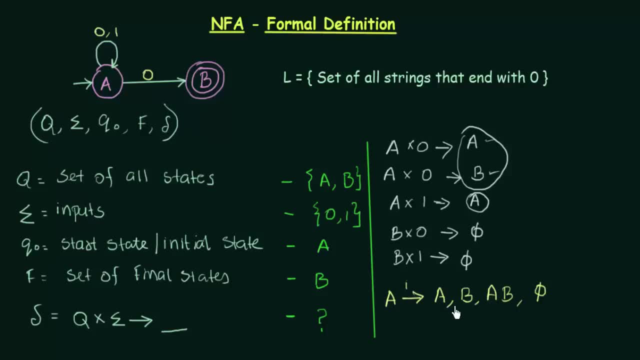 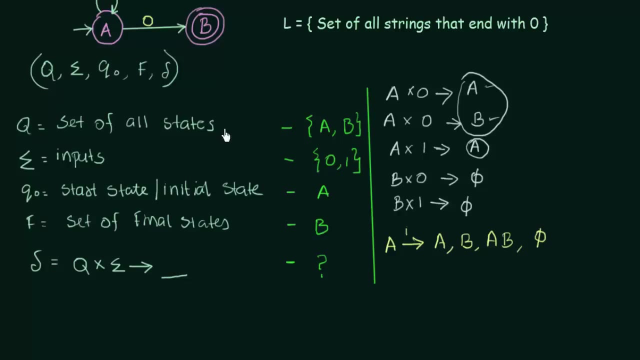 So this A, on getting a certain input, it has these four possibilities. It could either go to A, B, AB or PHI, Right, so there are four possibilities. Now let us take another example. Let us say that we have three states. 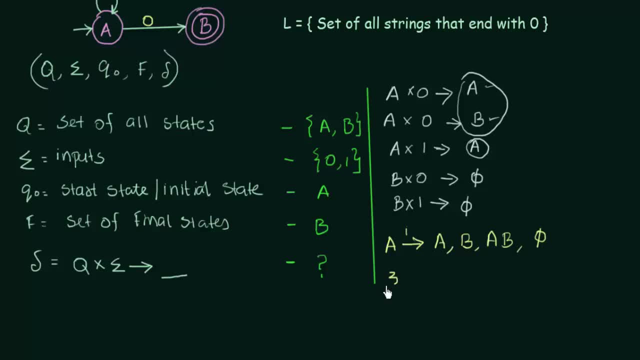 Suppose we have three states. Alright, we have three states which are A, B and C. Now in this example, suppose in state A we get a particular input. So what are the possibilities to which A can go? A can either go to A itself, it can go to B, or it can go to C. 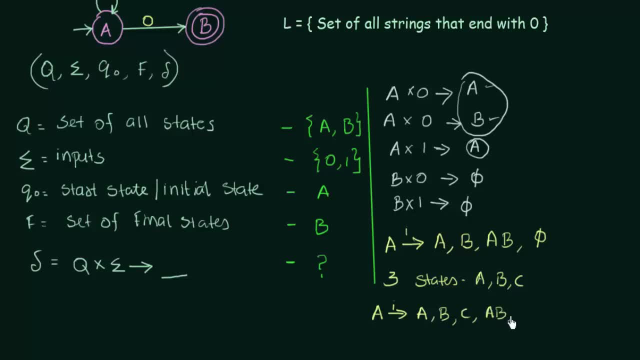 Or it can go to A and B Right, or it can go to A and C, Or it could go to B and C, Or it could go to all of them- A, B and C- Or it could not go anywhere. 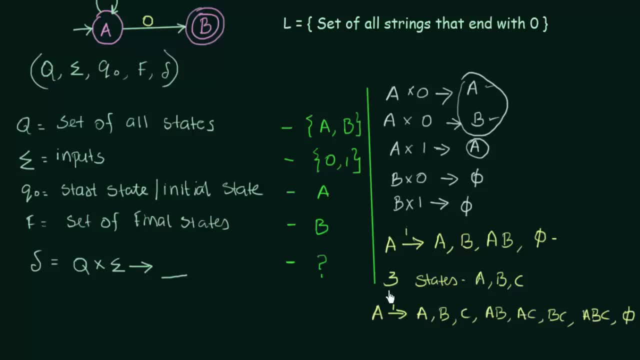 It could go to PHI. Okay, so we see that when there were three states, we had eight possibilities. When we had three states, there were eight possibilities: 1, 2, 3, 4, 5, 6,, 7, 8..